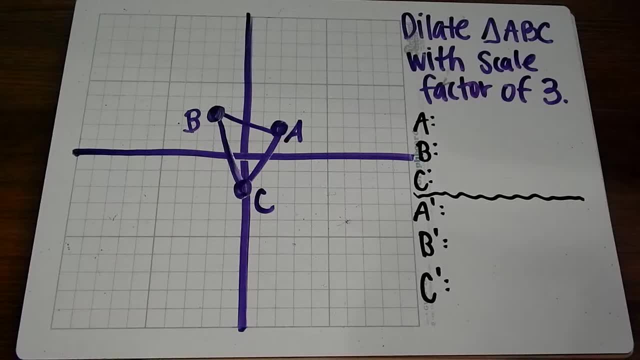 So when we dilate, if we have a scale factor greater than 1, our image is going to be enlarged. It's going to get bigger. If our scale factor is less than 1, it's going to decrease in size. It's going to get smaller. So the first thing we want to do here is list out each point: A, B and C. 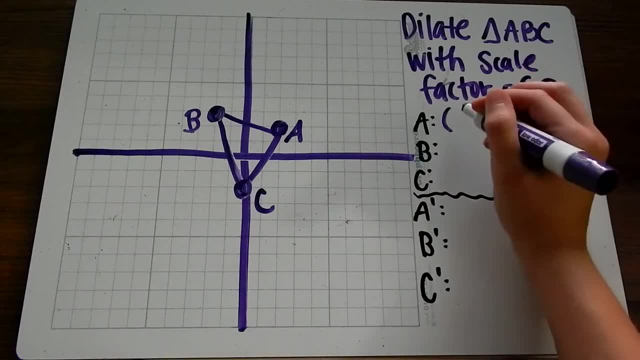 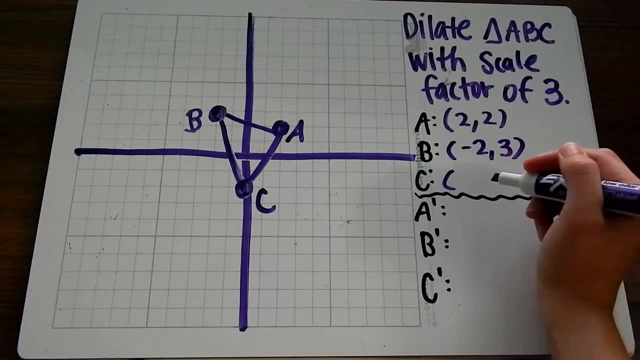 The coordinates for each point. So point A is 2, 2.. Point B is 2, 2.. Point C is 2, 2.. Point B is negative 2, 3.. And point C is 0,, negative, 2.. 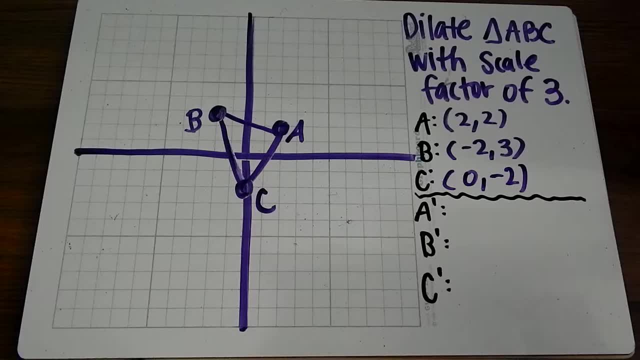 So now we want to dilate with a scale factor of 3.. All that means is multiply every point by 3.. That's all we're going to do. So to get A prime, we multiply 2 times 3,, we get 6.. 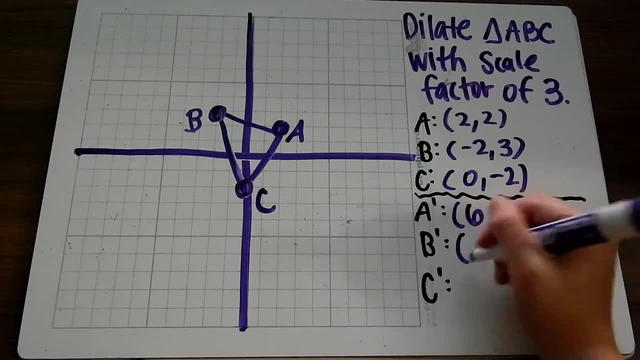 2 times 3, we get 6 again. For B: prime: negative 2 times 3 is negative 6.. 3 times 3 is 9.. And for C prime 0 times 3 is 0. So that's going to stay 0.. 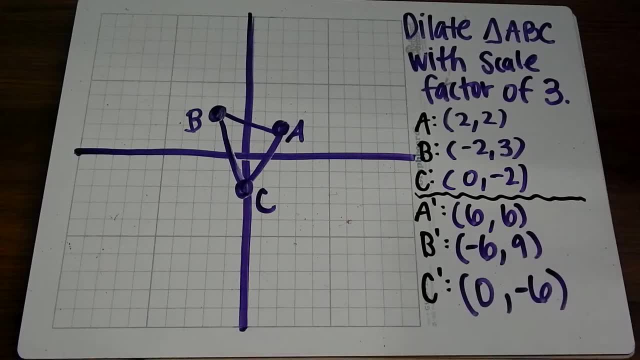 Negative 2 times 3 is negative 6.. Now we just have to plot our new points and we have dilated our triangle. So new A prime is going to be 6,, 6, which is here. That's A prime. 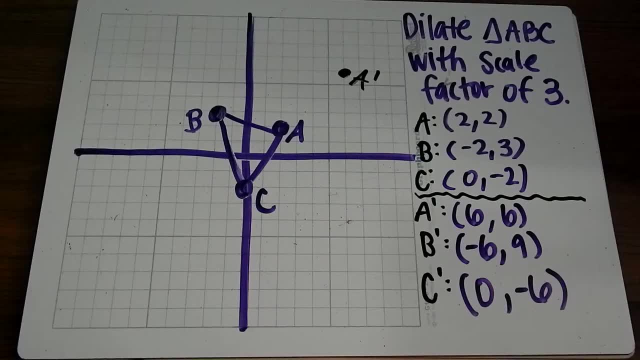 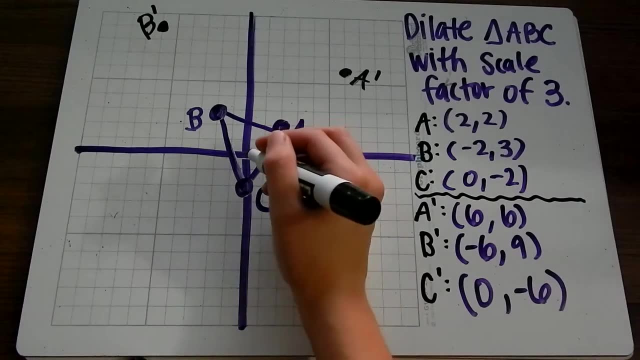 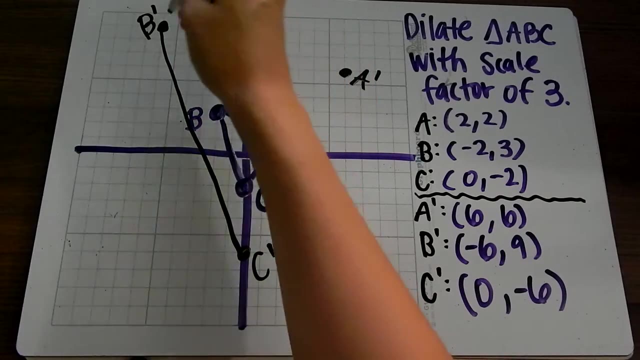 That's A prime. B prime is negative 6, 9,, which is right here. That's my new B. And C prime is 0, negative 6,, which would be here. That is C prime, And so I can now connect my dots. 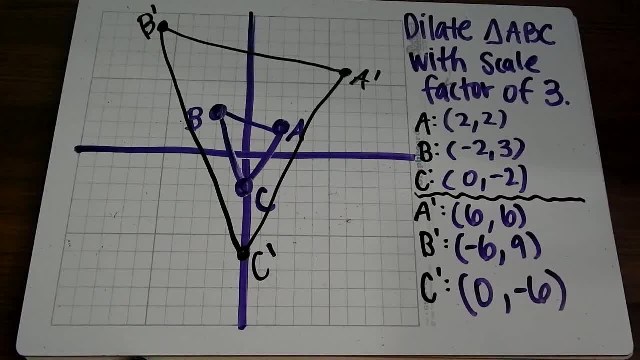 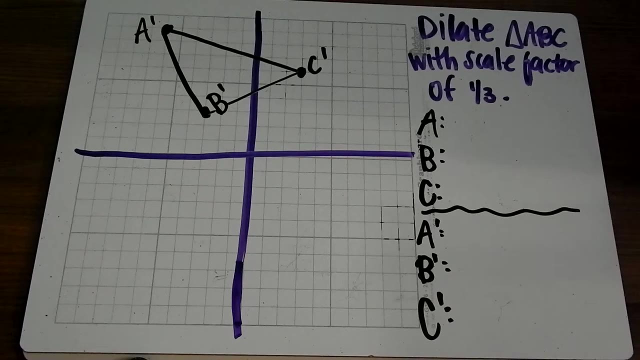 Draw my new triangle. As you can see, our triangle is bigger. It's actually 3 times bigger than our original triangle. For our last example, we are going to dilate with a scale factor of 1 third. Now we're going to do this the same way by multiplying the coordinates. 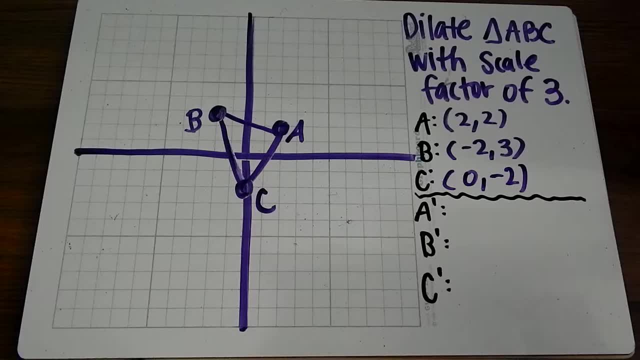 So now we want to dilate with a scale factor of 3.. All that means is multiply every point by 3.. That's all we're going to do. So to get A prime, we multiply 2 times 3,, we get 6.. 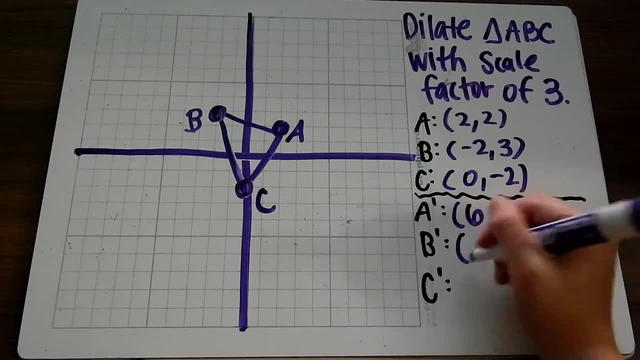 2 times 3, we get 6 again. For B: prime: negative 2 times 3 is negative 6.. 3 times 3 is 9.. And for C prime 0 times 3 is 0. So that's going to stay 0.. 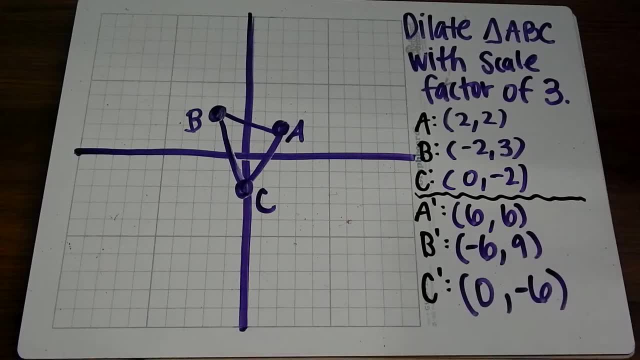 Negative 2 times 3 is negative 6.. Now we just have to plot our new points and we have dilated our triangle. So new A prime is going to be 6,, 6, which is here. That's A prime. 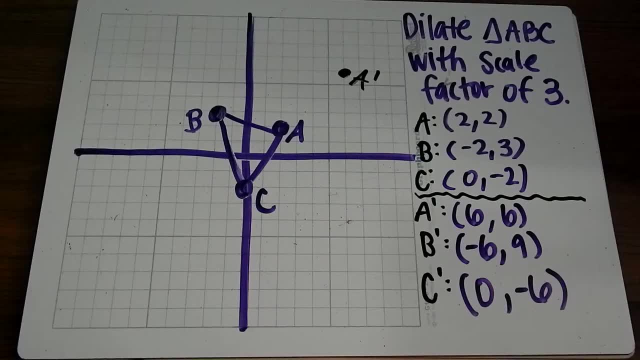 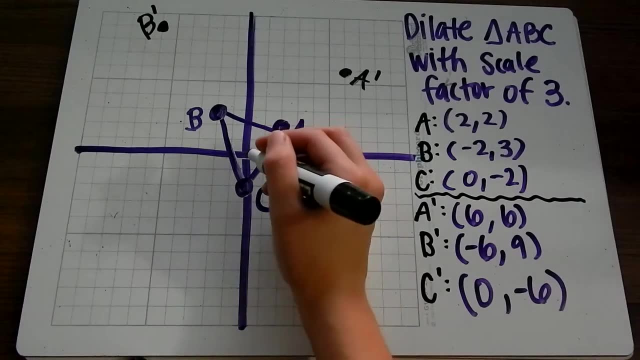 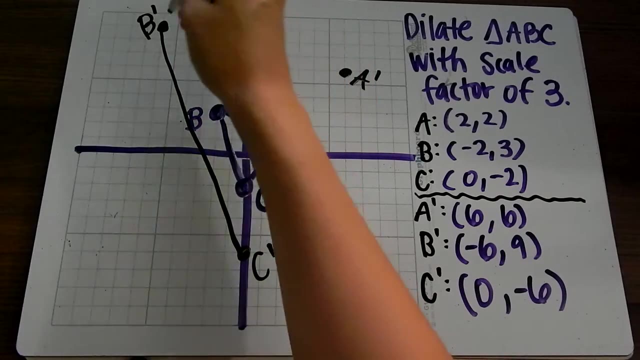 That's A prime. B prime is negative 6, 9,, which is right here. That's my new B. And C prime is 0, negative 6,, which would be here. That is C prime, And so I can now connect my dots. 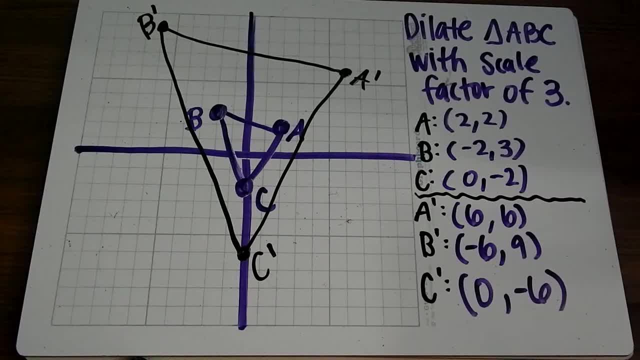 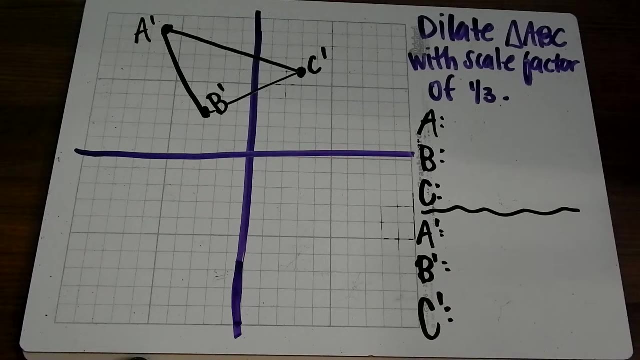 Draw my new triangle. As you can see, our triangle is bigger. It's actually 3 times bigger than our original triangle. For our last example, we are going to dilate with a scale factor of 1 third. Now we're going to do this the same way by multiplying the coordinates. 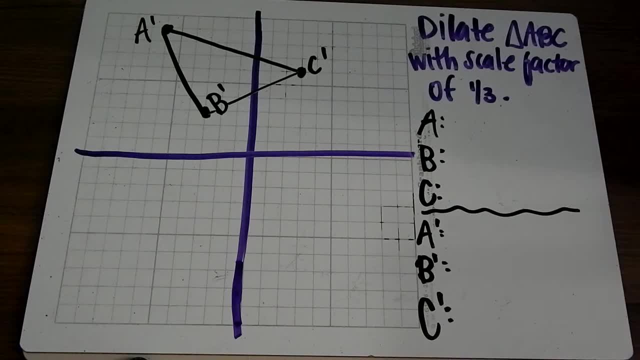 However, since our scale factor is less than 1, our triangle is not going to get bigger, it's going to get smaller. So let's list out the points for A, B and C, just like we did last time. Okay. 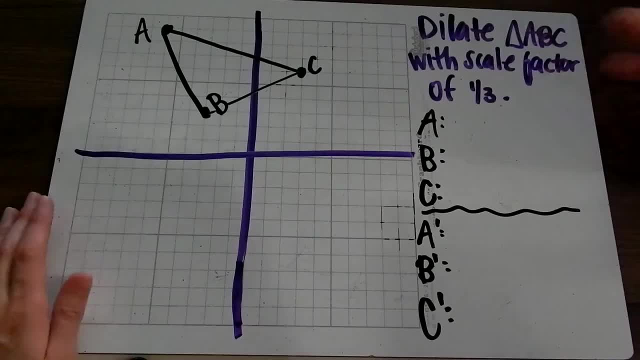 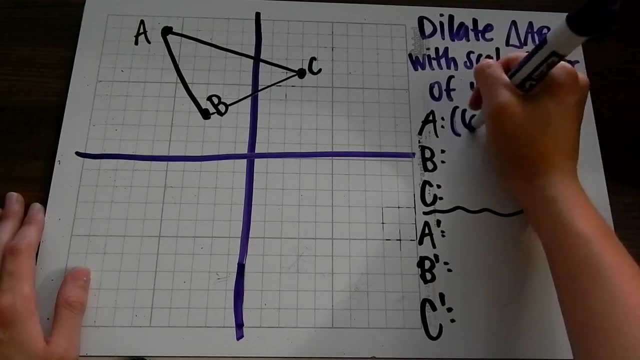 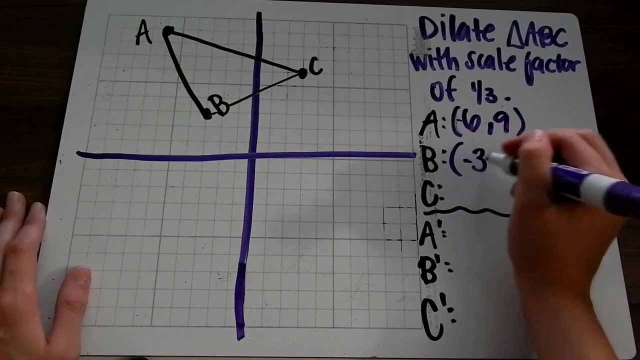 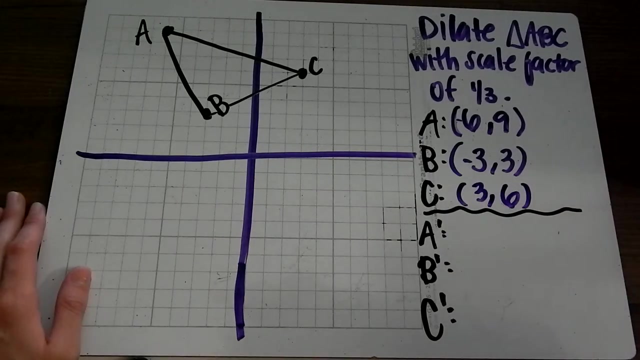 These are not prime, those are just regular a, b and c. So our point a is going to be, Point b is and c is. So negative 6, positive 9, negative 3, 3, and 3, 6 are our points. 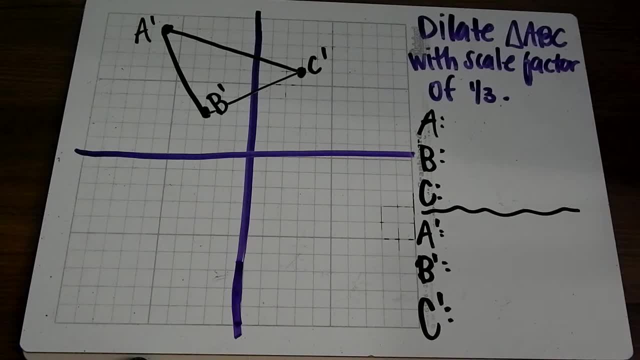 However, since our scale factor is less than 1, our triangle is not going to get bigger, It's going to get smaller. So let's list out the points for A, B and C, just like we did last time. These are not prime, those are just regular a, b and c. 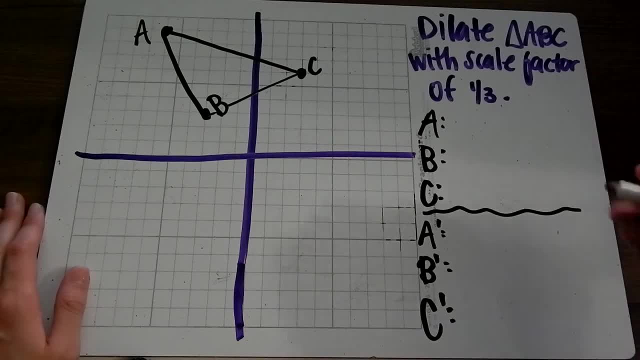 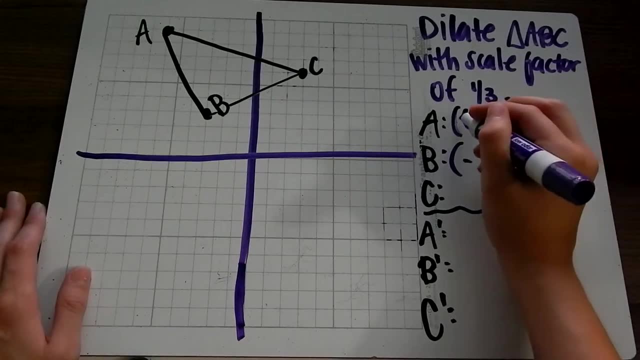 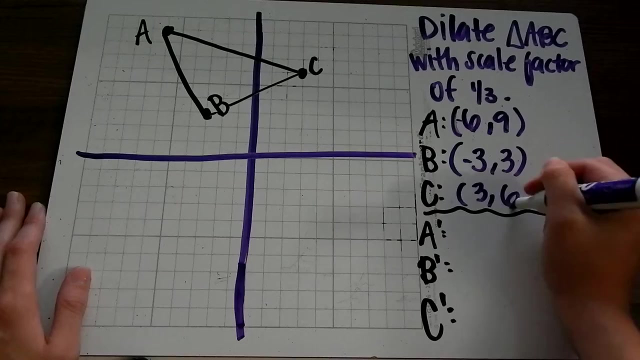 So our point a is going to be 6, 9.. Point b is negative, I'm sorry. negative 6, 9,, negative 3, 3.. And c is positive 3, 6.. So negative 6, positive 9, negative 3, 3, and 3, 6 are our points. 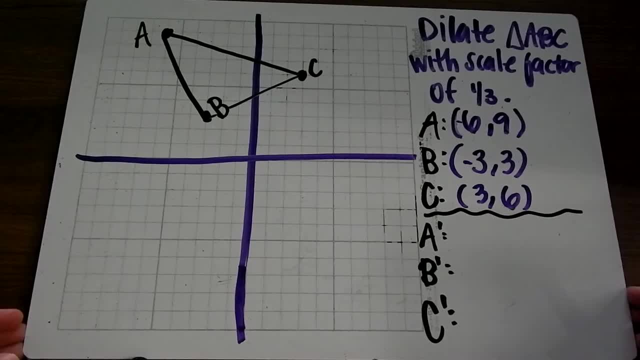 So, since we have a scale factor of 1 third, all we're going to do is multiply each point by 1 third, each x and y. So negative 6 times 1 third. when you multiply by 1 third, you're actually just dividing by 3.. 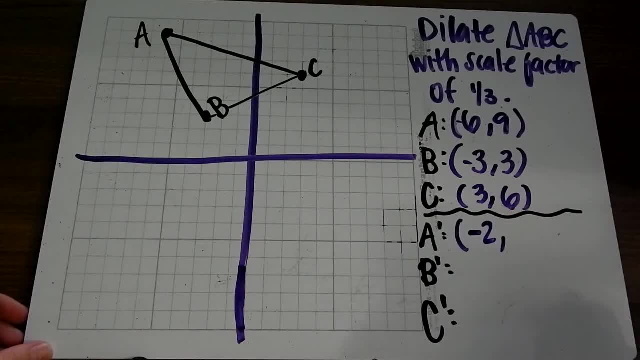 So: negative 6 times 1 third is negative: 2.. 9 times 1 third is 3.. Again, just dividing by 3.. Negative 3 times 1 third is negative: 1.. 3 times 1 third is 1.. 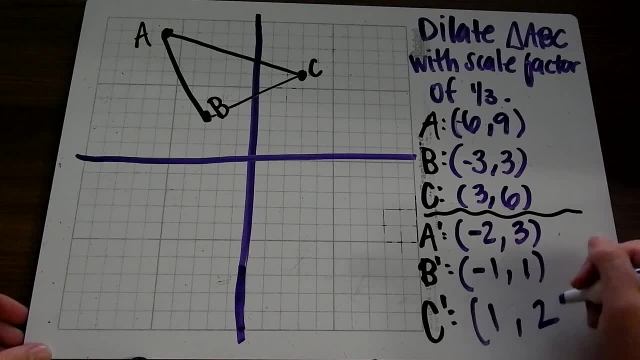 3 times 1 third is 1.. And 6 times 1 third is 2.. Now I can go ahead and make my new points and draw my new triangle based on those coordinates. So a prime is negative 2, 3.. 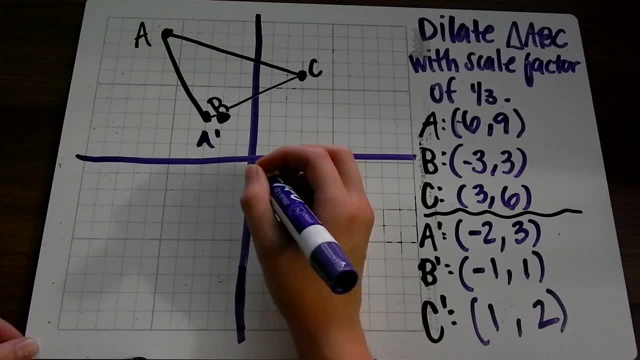 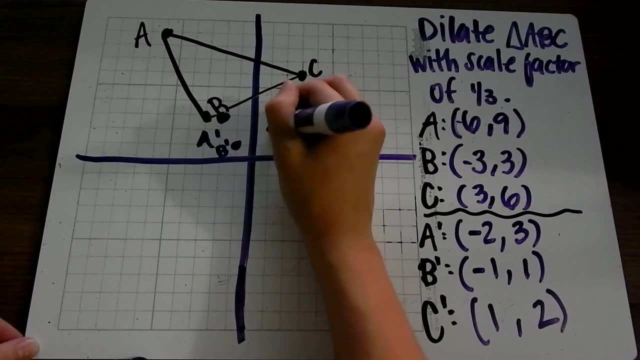 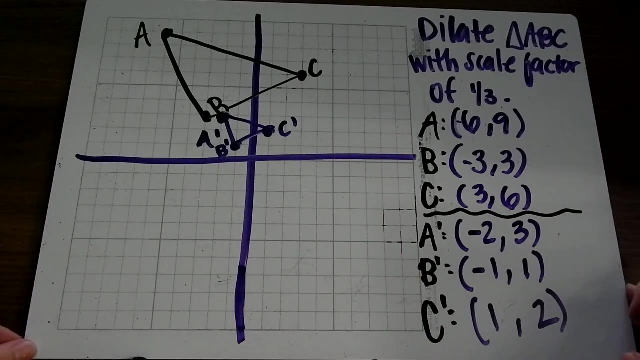 It's going to be right. here, b prime is negative 1, 1.. Right here, c prime is 1, 2, which is right here. As you can see, the triangles look the same. One's just a lot smaller, which is what we want. 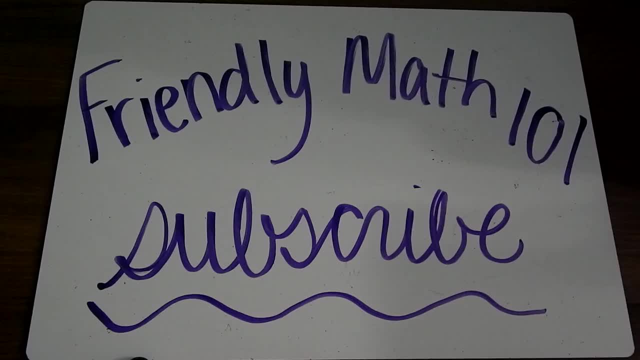 Thank you for watching And for more math tutorials, please subscribe to our channel, Friendly Math 101..